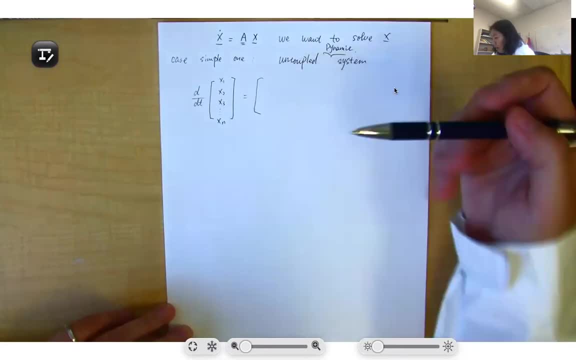 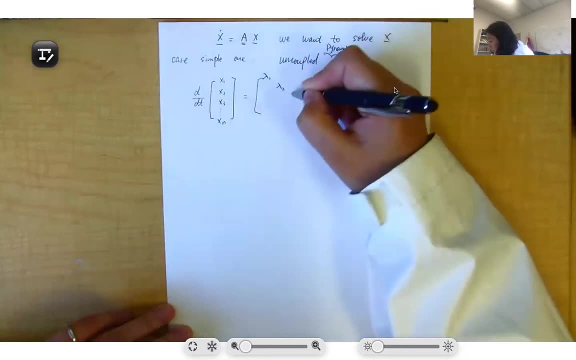 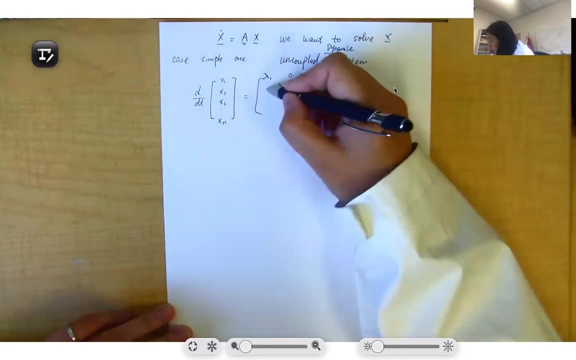 So that the coefficients won't influence each other. That means we will have a diagonal matrix, So lambda 1, lambda 2, lambda 3, dot, dot, dot to lambda n And all the other side will be zero. This will be zero. 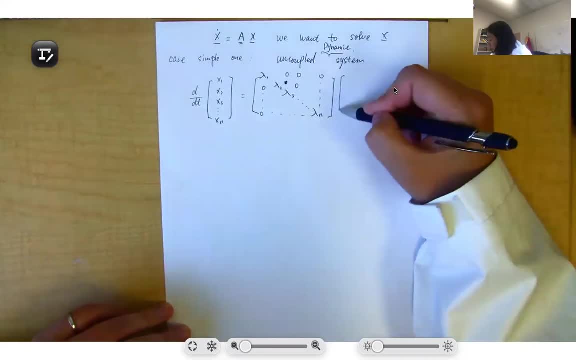 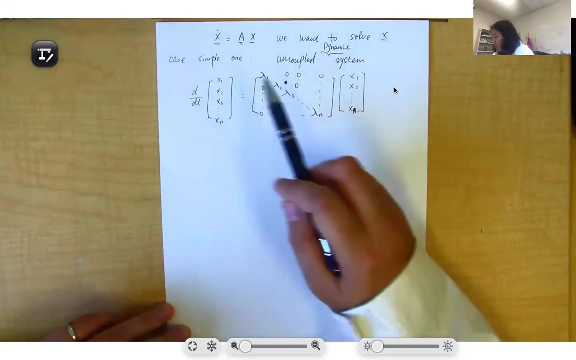 And this is a diagonal matrix And times itself x1, x2, dot dot to xn And you can see that basically the x1 differentiate is time will be equals to lambda x1. And it won't be related to x2 to xn. 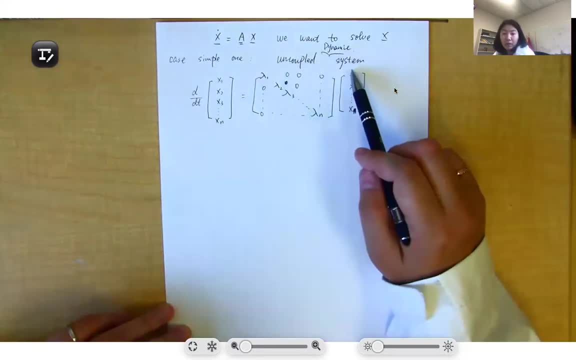 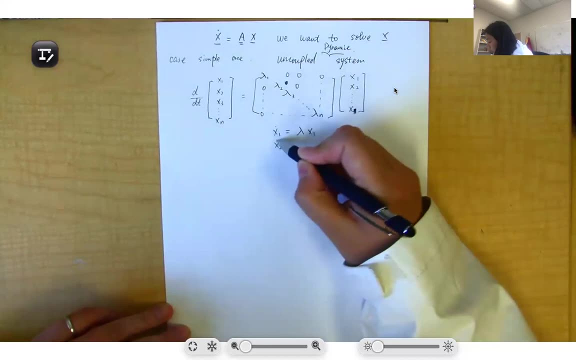 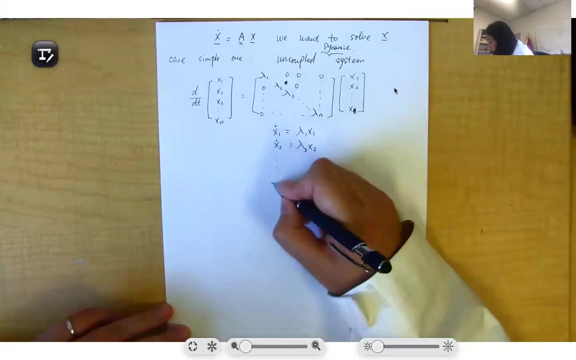 So we call it uncoupled dynamic system, which is very simple. So x1 dot will be equals to lambda x1.. x2 dot will be equals to lambda x2.. 1,, 2.. Until, xn dot will be equals to lambda n xn. 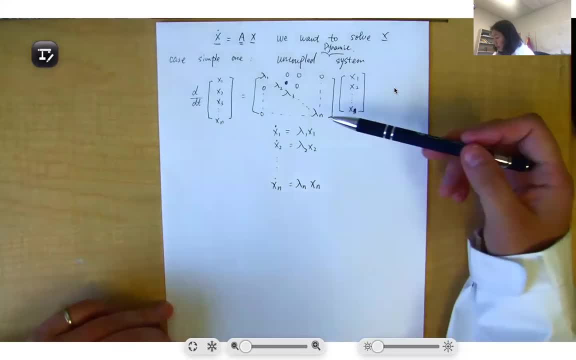 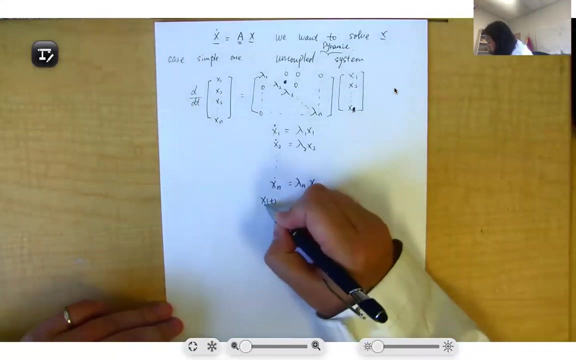 Okay, So we know that this is ordinary differential equations with constant coefficients, So that the solution format will look like the explanation. So our solution will look like: xt or nt will be e to the lambda, nt to x to some constant, some constant, cn, some constant. 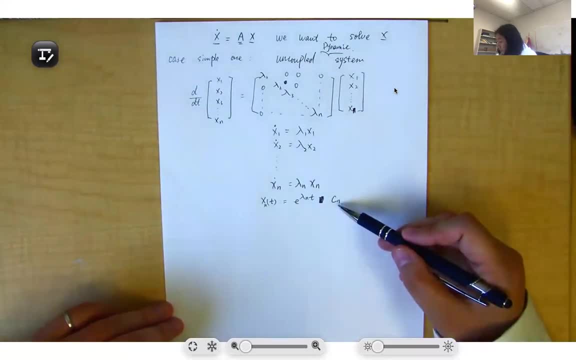 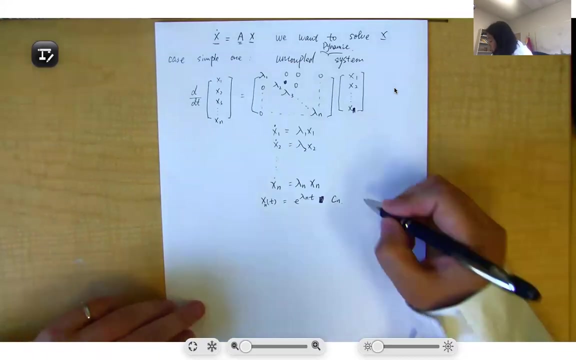 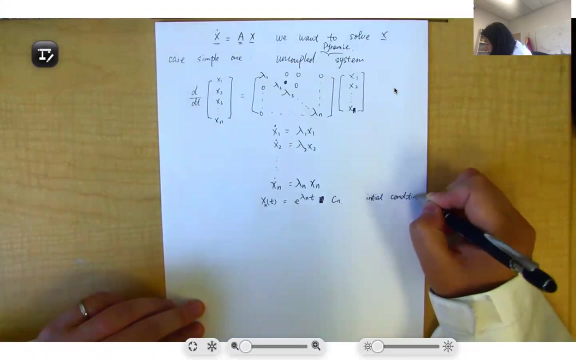 So the solution format will be decided by the conditions of whatever It can be initial value conditions, It can be boundary value conditions. So if we give an initial condition, basically at time equals to zero, you will have x, 1, 0.. 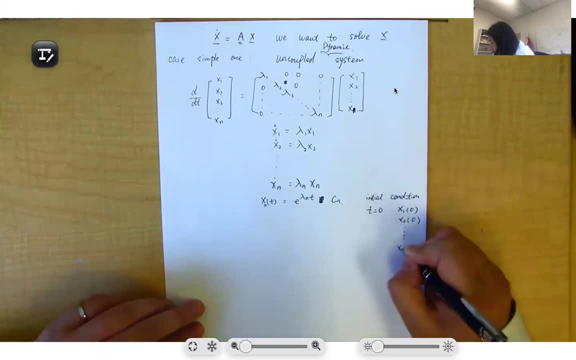 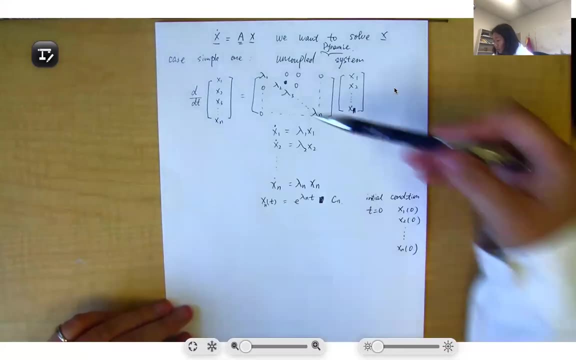 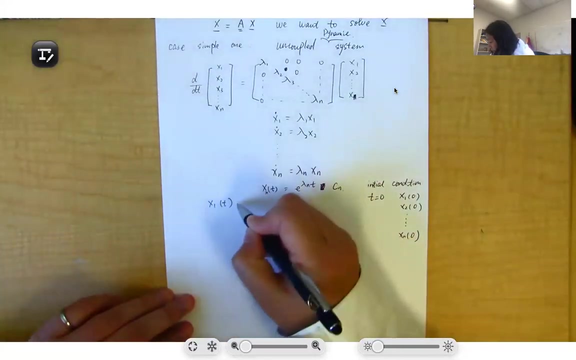 x2, 0.. Until xn 0.. For this nth order ODE right. So you will have n conditions to make sure your x1, x2, until xn. Then our final solution will look like: x1t equals to e, to the lambda 1t. 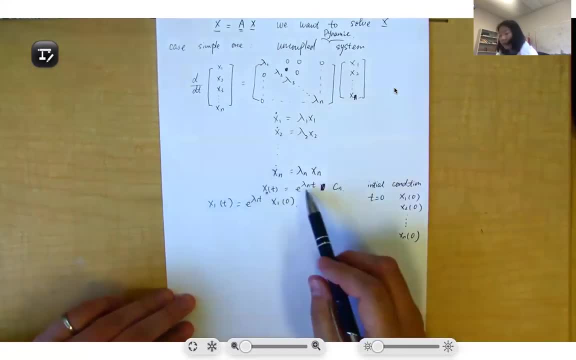 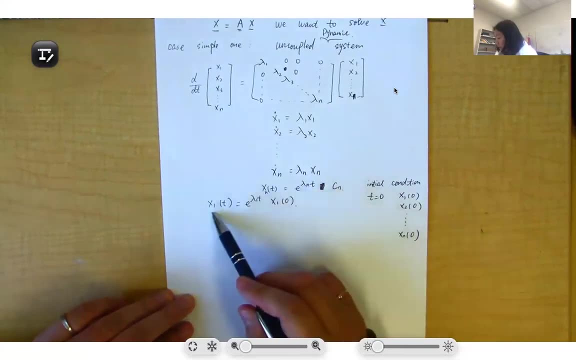 Cn will be just x1, 0. We call e to the lambda 1t. So if x1t equals to 0, then this will be just 1.. So that x1t equals e to the lambda 1t, x1t. 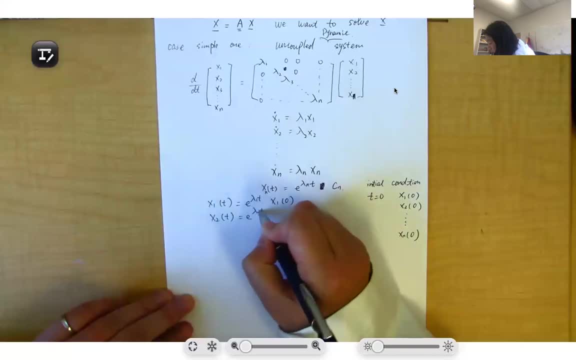 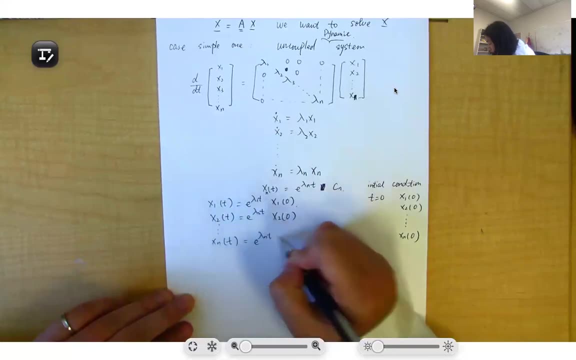 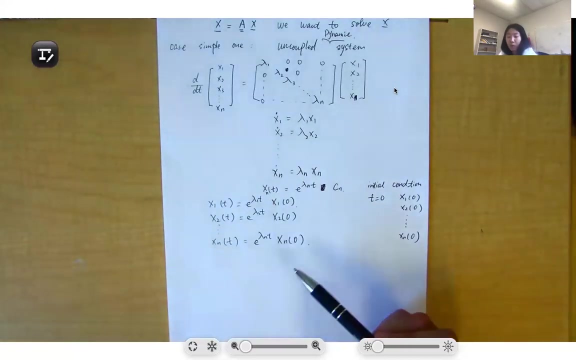 x2t will be equals to e to the lambda 2t, x2, 0.. Until you have xn, t will be e to the lambda nt xn- 0.. Okay, And you can rewrite this solution format to be matrices. 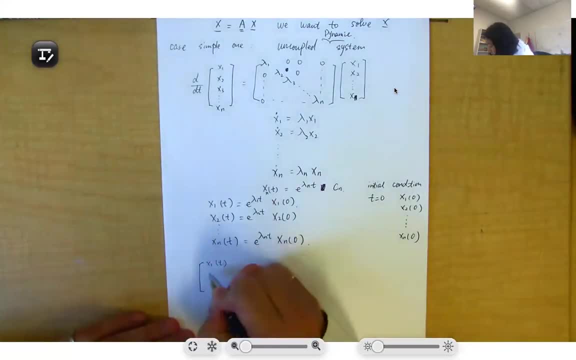 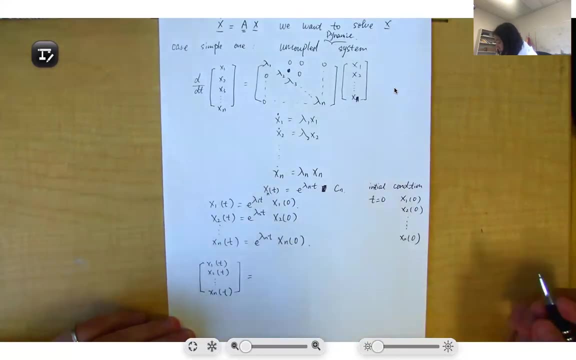 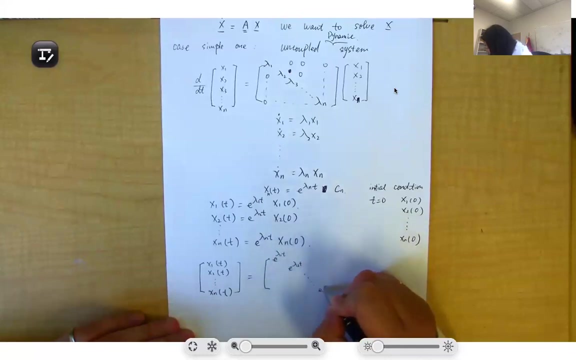 There you have it. You have x1t, x2t until xn. t will be equals to e to the lambda 1t, e to the lambda 2t until e to the lambda nt Times. so all this part will be 0.. 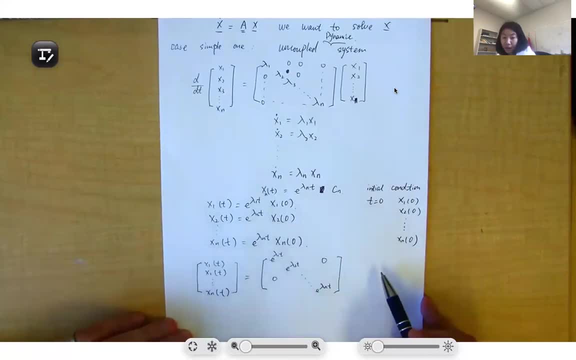 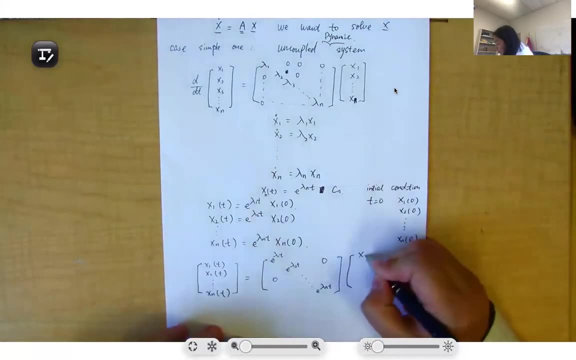 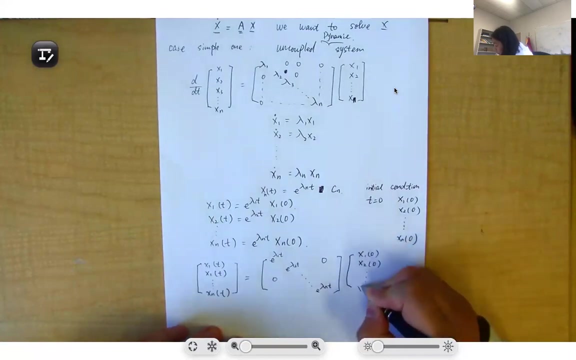 This is a diagonal matrices because they are uncoupled. They are now influencing each other from x1 to xn, So that this part will be u initial condition: x1, 0,. x2, 0,. double down to xn. 0. 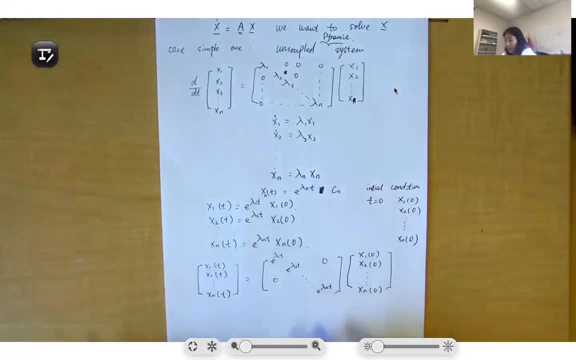 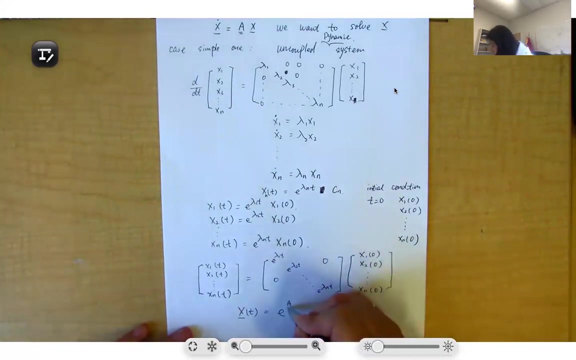 Okay, Then the final solution for this uncoupled system will be x. This is a 1d vector, xt will be e. to the this matrices, the diagonal matrices, We can say a, t, t, x, 0.. 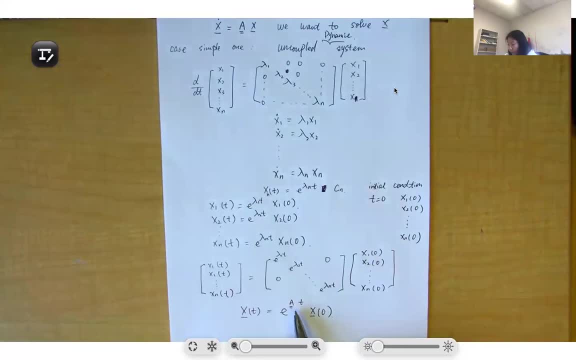 And you know this: a is a diagonal matrices for this system because they are uncoupled. Okay, So that is valve b, using matrices to represent the ordinary differential equations. Then our next question is that you know this: a is uncoupled. 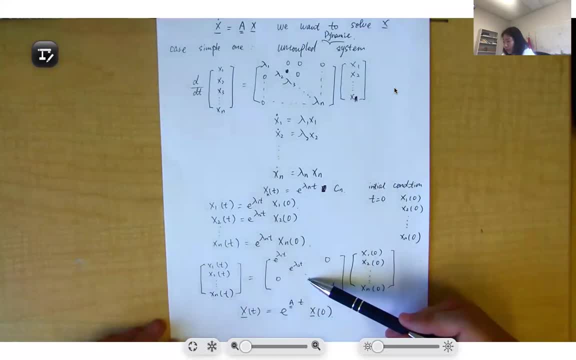 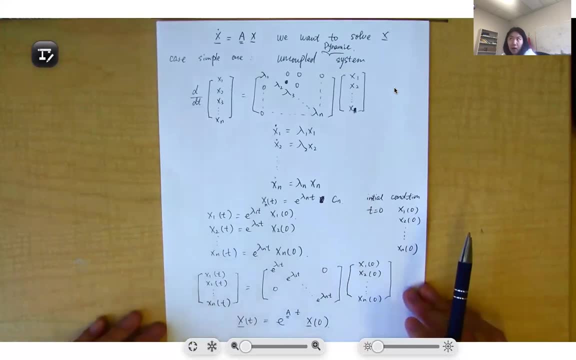 This is an uncoupled system here, So this is a diagonal matrices. What if they are coupled? Then things can be complicated. Can we use eigenvalue and eigenvectors to simplify our coupled dynamics to be uncoupled dynamics? Okay, 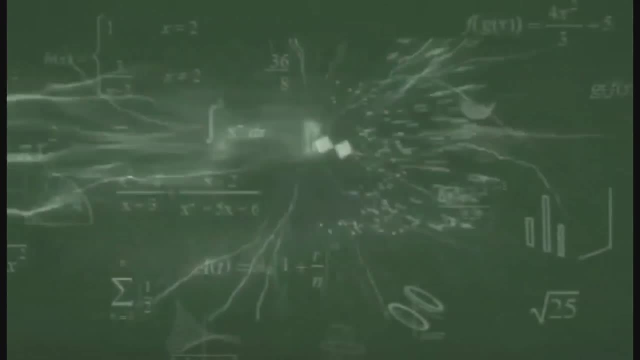 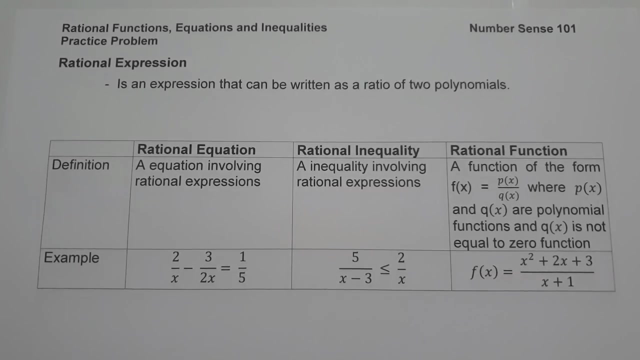 In today's video we are going to have a basic introduction on how to determine whether the given is an example of rational functions, rational equations and rational inequalities. But let us define first what is a rational expression. So when we say rational expression, 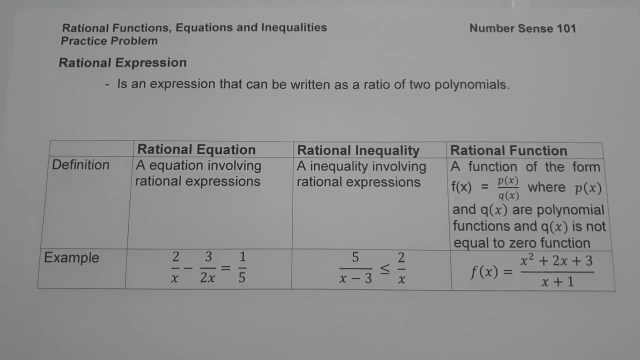 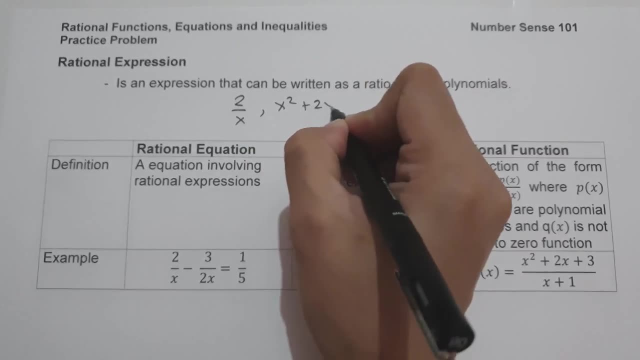 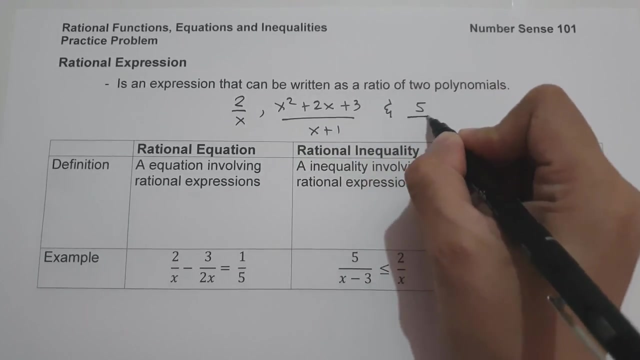 it is an expression that can be written as a ratio of two polynomials. For example, let's say we have 2 over x, x squared plus 2x plus 3, all over x plus 1.. Let's say we have 5 over x minus. 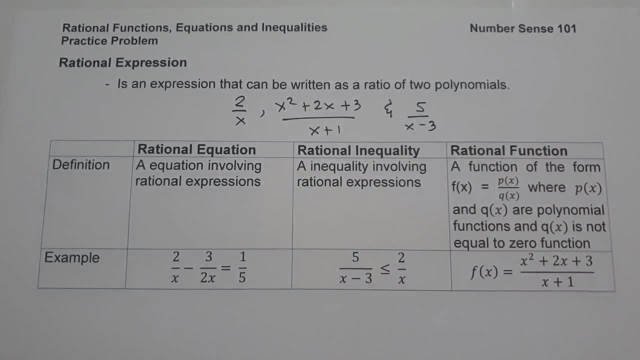 3.. So those are the examples of rational expression, because they are written in the ratio of two polynomials. Now let us define what is a rational equation: rational inequality and rational function. So when we say rational equation, it is an equation involving rational 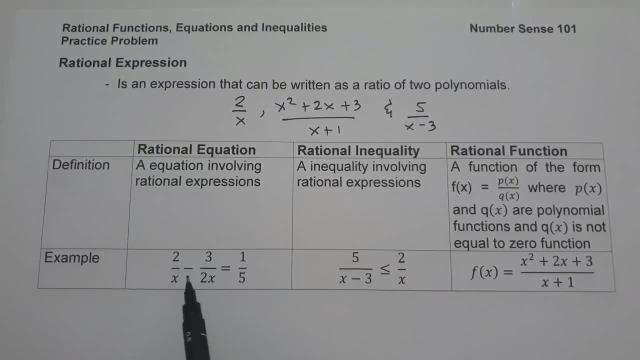 equation. So when we say rational equation, it is an equation involving rational equation. For example, 2 over x minus 3 over 2x equals 1 over 5 is an example of rational equation. And when we say rational inequality, it is an equality involving rational expression. 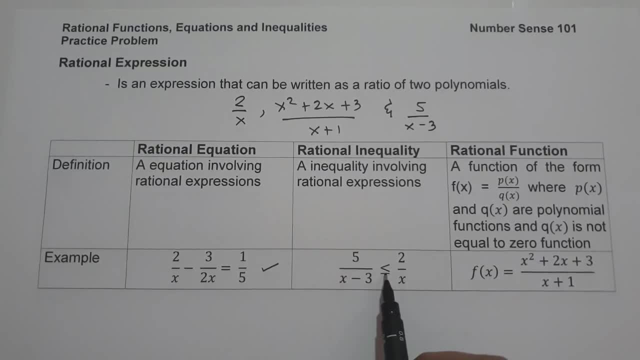 So we have 5 over x minus 3, less than or equal to 2 over x. So this one is an example of rational inequality and the inequality symbol is less than or equal to. So whenever you have an inequality symbol, the given example is rational inequality. And lastly, we have rational function. So when